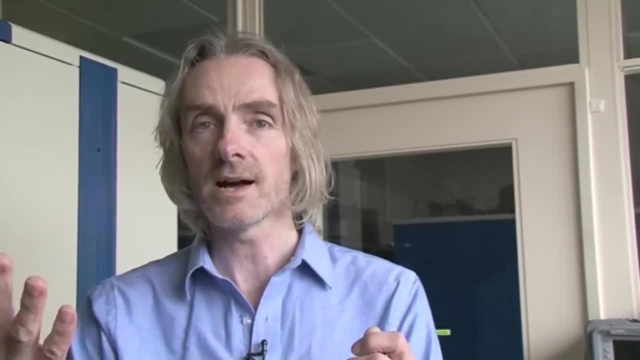 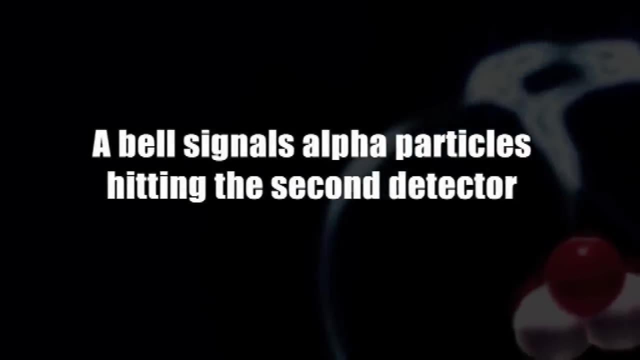 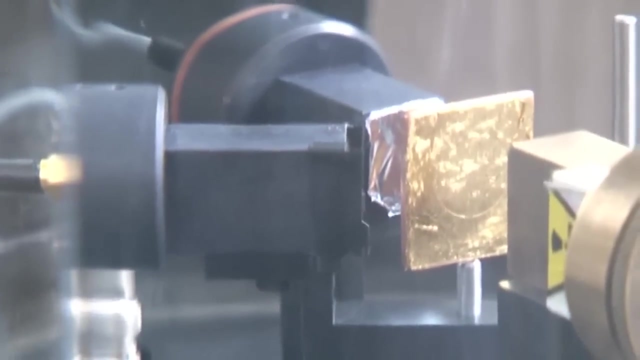 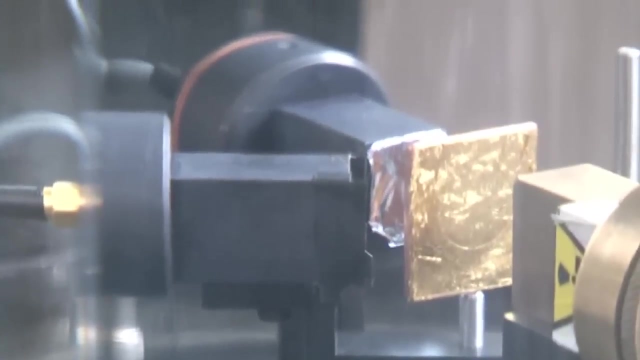 room. They were holding a tiny fluorescent screen and looking just by eye for flashes of light on the screen. We have replicated that with modern detector technology. In its current position behind the foil it will measure one count every few seconds. As Rutherford deduced, most of the gold atoms empty space, So the alpha particles are still. 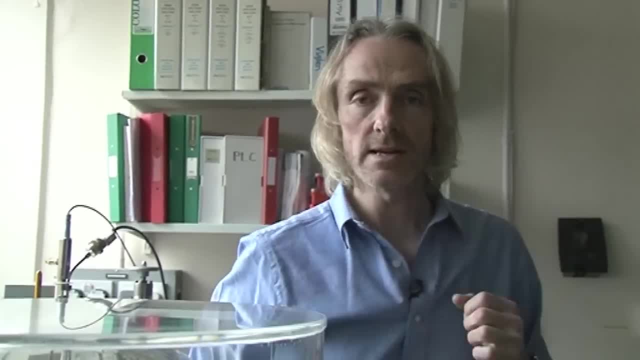 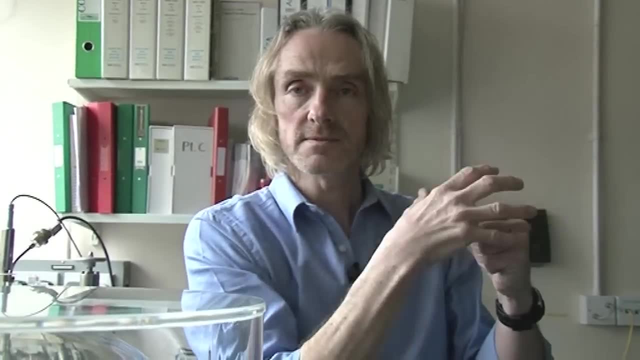 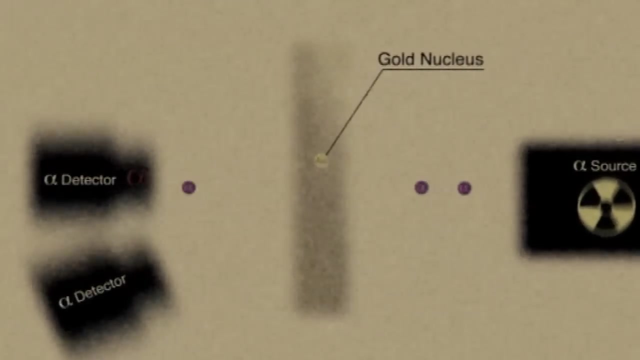 that just goes straight through, doesn't see anything and goes through in a straight line. Occasionally one of the particles will come close enough to the nucleus of the gold atom that it will be deflected by the electric field from the positive nucleus. If it comes at a glancing blow it will be deflected through a small angle. 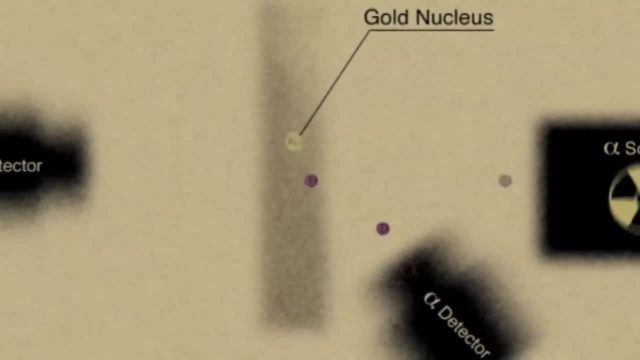 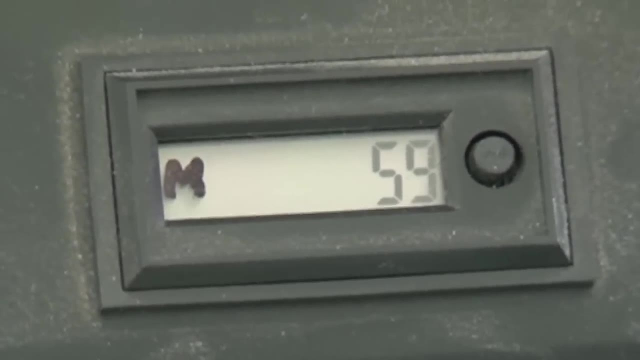 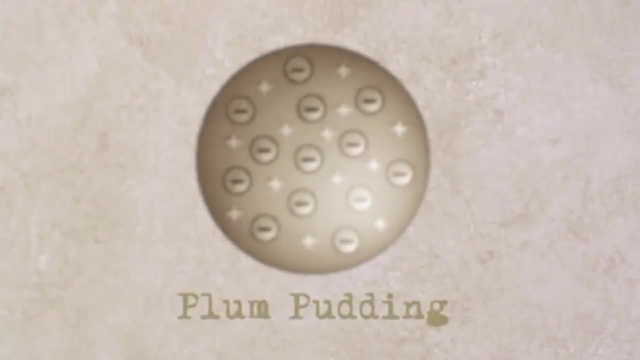 If it hits it head on, it will just bounce straight back And it's fascinating, I think, to them that this was telling us something very important that we didn't know about the very deep structure of matter. It showed that the atom had a heavy nucleus with mostly empty space. 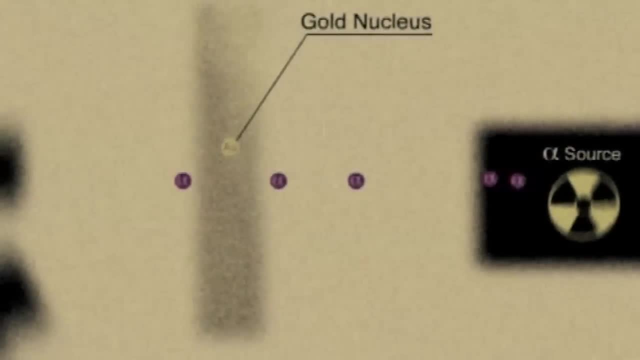 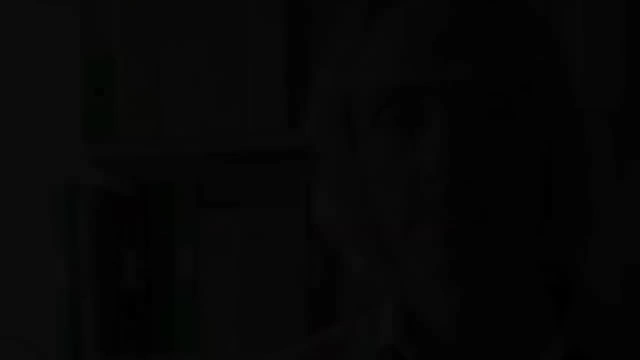 with electrons distributed around it, which is exactly the picture we now have. It was also the start of particle physics. What Rutherford was doing and what we're doing here is taking a beam of particles, firing it at a target, looking at the way the particles are scattered. 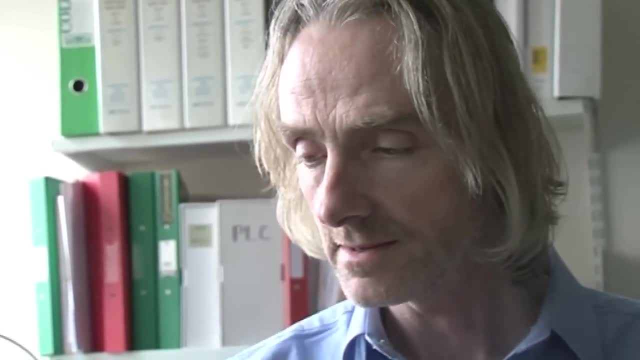 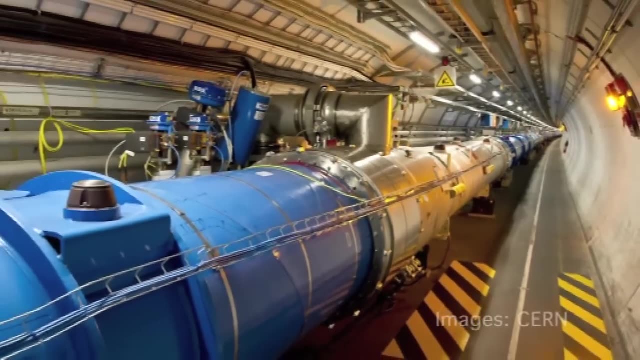 and from that deducing what was going on inside the target And 100% of the time, 100 years ahead. we now have the Large Hadron Collider, where we do the same thing: We fire a beam of particles at a target. In that case, the target is another beam coming the other way. 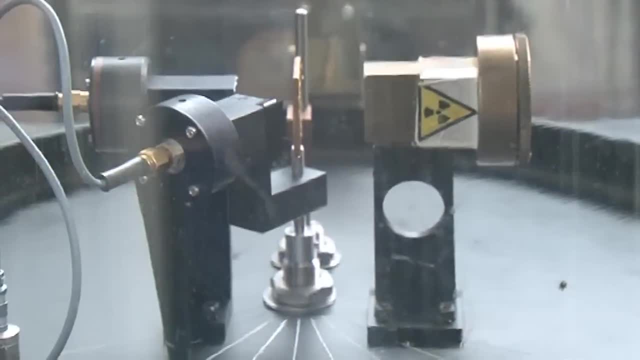 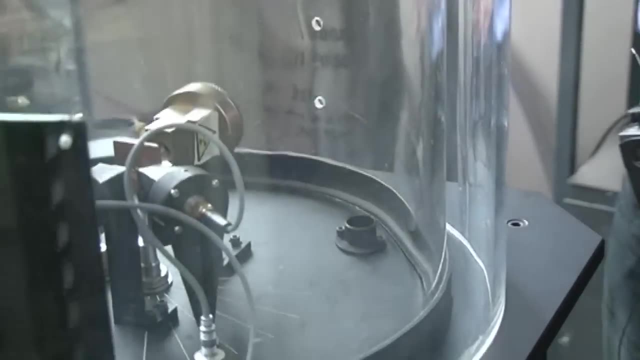 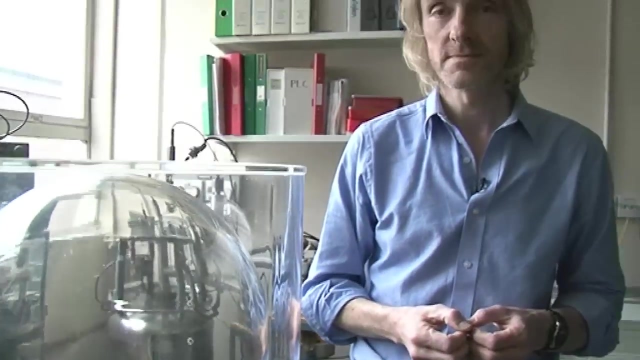 We look for the particles being scattered out of that collision process and try to deduce what was going on in the collision from the behaviour of the scattered particles. And all that comes from Rutherford's original idea of firing a beam at a target. So in a century we've come from an apparatus that would fit on the desk. 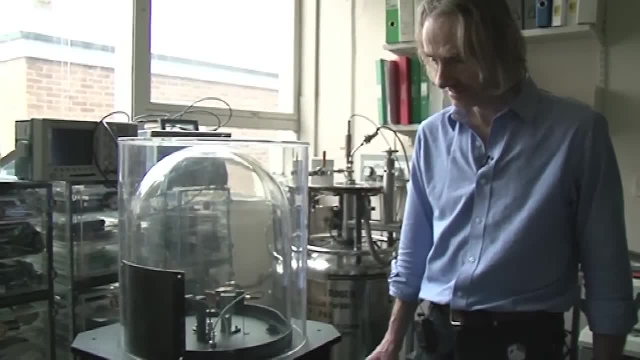 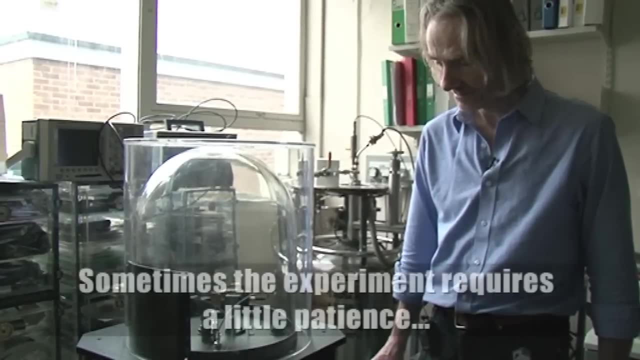 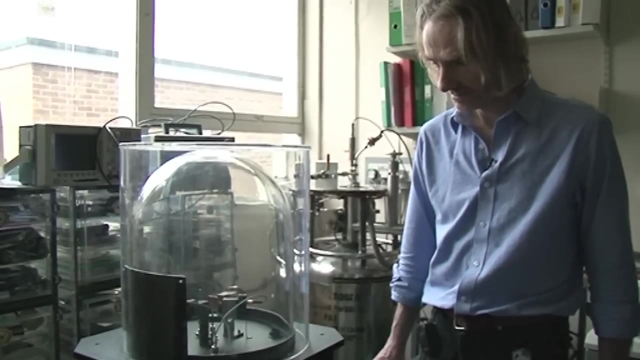 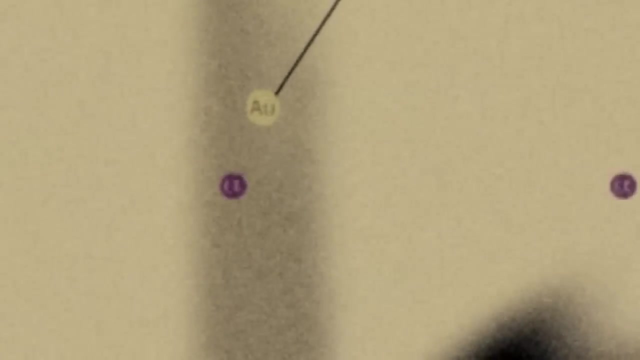 that was the cutting edge of physics- to the Large Hadron Collider, which is 27 kilometres in circumference. What was happening was that the alpha particles were going through and missing the nucleus, because the nucleus is extremely small and the atom, by comparison, is very big.